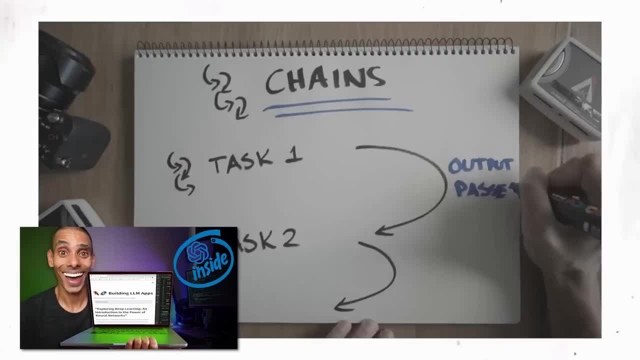 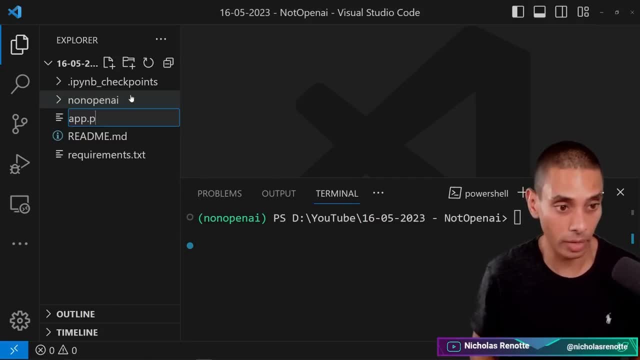 This will allow you to interact with the different LLM models through a simple user interface. We're going to blast through this pretty quickly, because it's pretty similar to what we did inside of the Langchain crash course. In the Langchain crash course, we started out by creating a file called apppy. 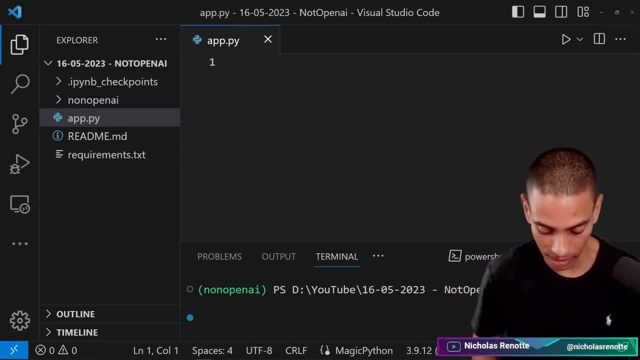 This is where our LLM application is going to live. Now, the first thing that we need to do is import Streamlit, Streamlit, Streamlit as st. This is going to give us our app development framework. Let's add a comment. 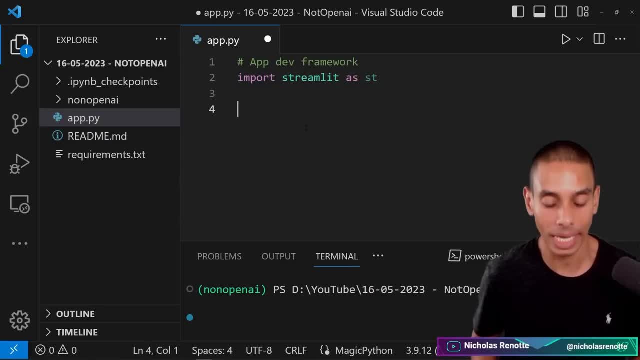 App dev framework. And then what we want to do is have a title, So we're going to say title- Actually we don't need to set it to a variable, So sttitle. I'm going to plug in a emoji, because we've got to make it look sweet, and we're going 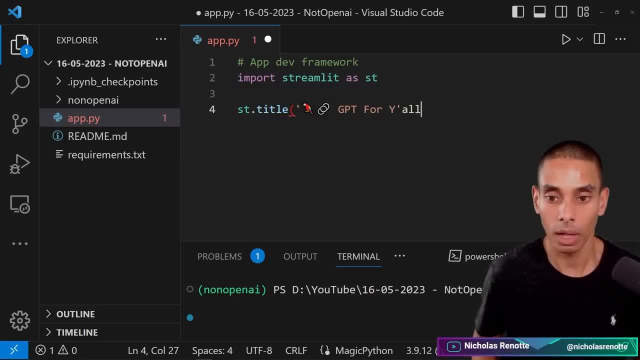 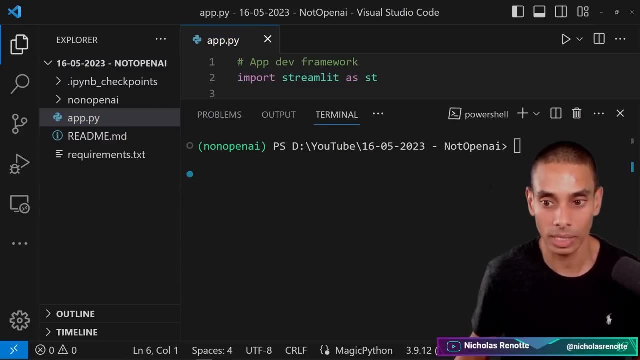 to title it GPT for y'all Y'all. We should probably escape that Perfect. All right, cool. So this is the title, and then what we want to do is let's start up our app, just to make sure this is working. 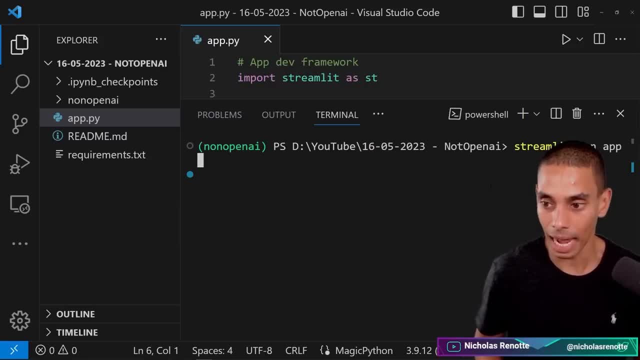 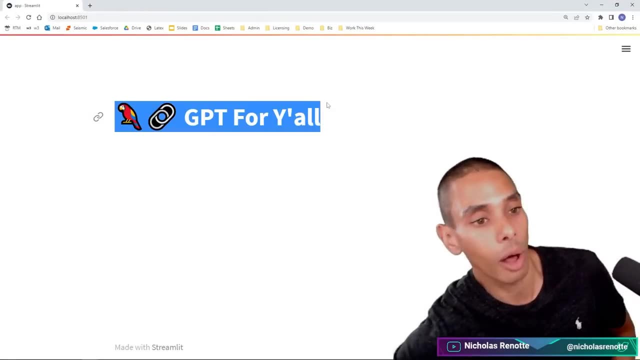 I can't imagine this is broken right now. So we can run Streamlit app or Streamlit run apppy. This will open it up in a new browser window. Perfect, So we've got GPT for y'all happening right now. So that is our title. 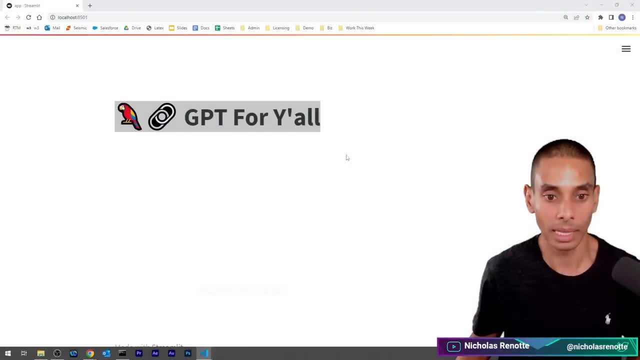 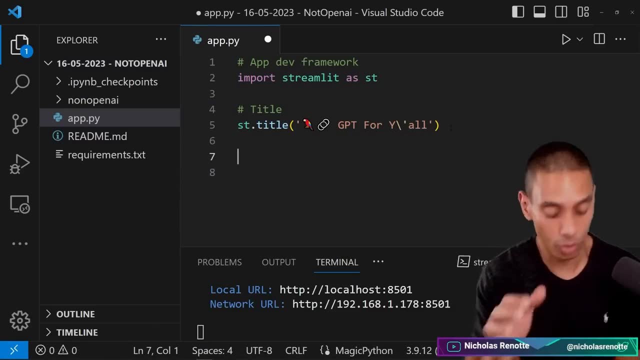 Now, if we wanted to change that, you could change it to whatever you want to do, something a little bit more appropriate for a business application. Okay, So that is our title. The next thing that we want to do is include a place that we can actually pass through. 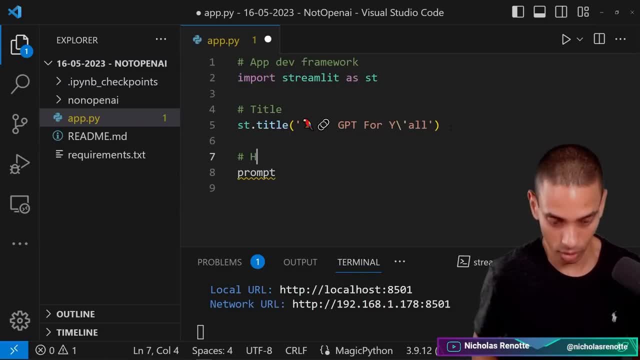 a prompt. So we're going to create a variable called prompt, So prompt holder. So this is the prompt. Okay, Text box, And we are going to set that equal to sttextinput. If you had bigger text inputs you might choose to go with text area. 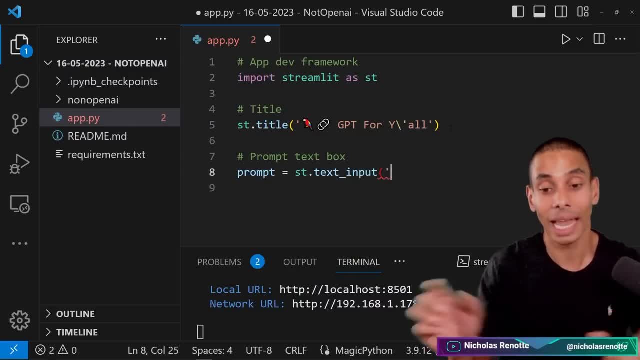 I found text input works pretty well And we are going to include the label for this. So we're going to say plugin. Let me make sure my head is not covering that. Now we're good Plug in your prompt here And if we go and save and we go and refresh our app again, take a look. 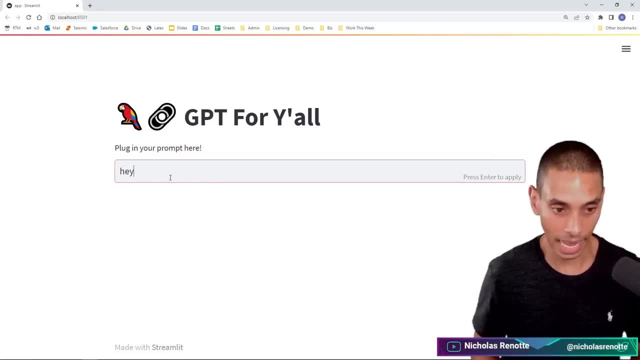 So we've now got somewhere that we can type in a prompt, right? So I could say, hey, how's it going? And eventually, when we hit enter on our keyboard, we want to do something. Right now it's not doing anything because, like you can see that I'm hitting enter. 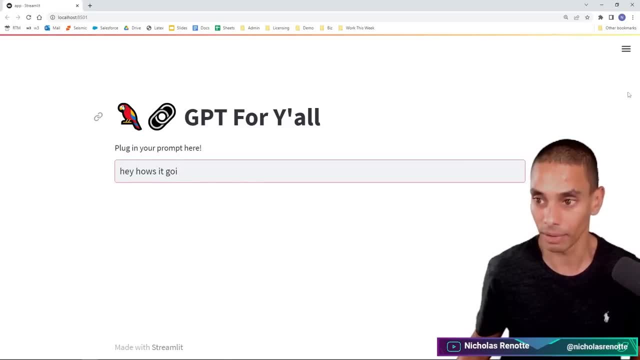 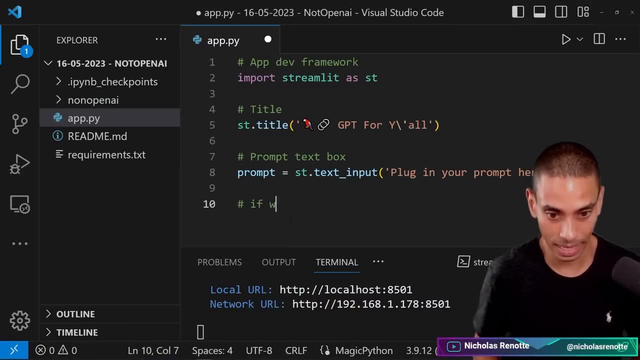 If I go and change it, if I hit enter, it's running up there. You can see it really briefly. right, We actually need to do something or activate a trigger once we go and hit enter, So relatively easily. So if we hit enter, do this. 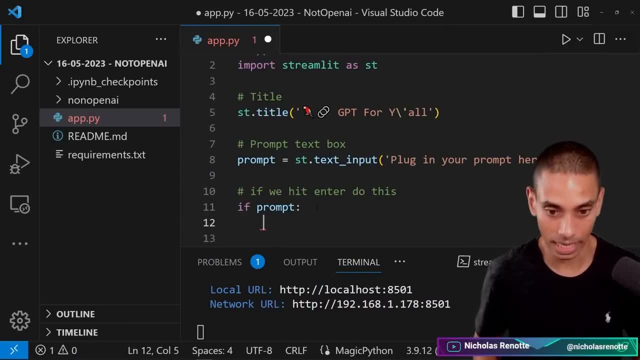 So we're going to say if prompt, and then all we need to do is right now- for right now we don't actually want to go and import anything- We'll get to that. So we're going to write stwrite and we're just going to write out our prompt, so we can. 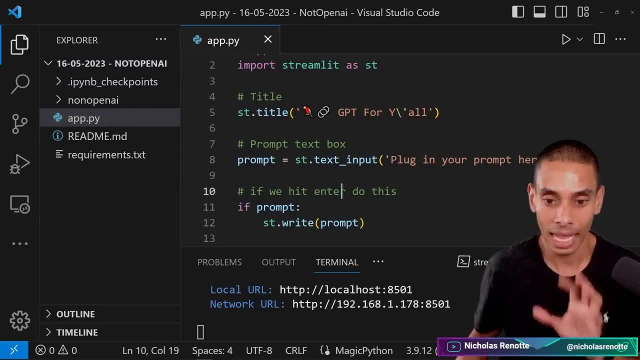 at least see that we're doing something. We're getting a little bit of feedback, So we're going to say, if we hit enter, then we're going to do whatever's here, right? So that is our baseline app. Let's just go and test it out. 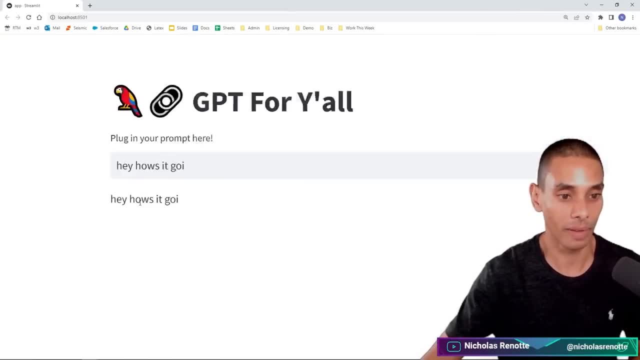 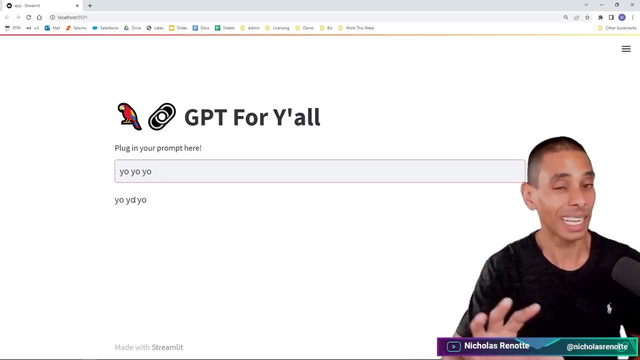 So if we go and refresh so you can see it's already printing out the output of our prompt there. So if I go and change it to yo yo yo, you can see that we are outputting the output there. That at least gives us the shell for our GPT for all app. 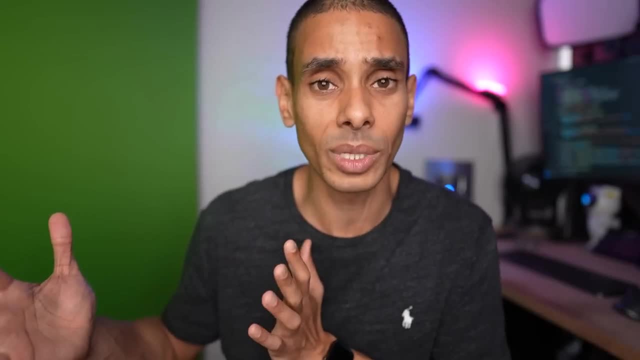 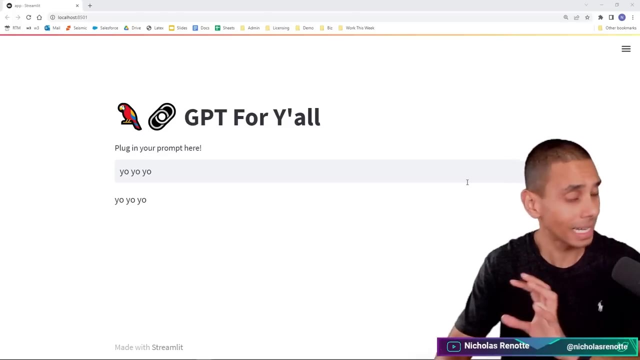 So we've got an app that we can interact with, but we haven't actually done any LLM stuff yet. Time to bring the thunder First up: importing language Langchain dependencies. So we've got the shell up and running, but right now we haven't actually done anything. 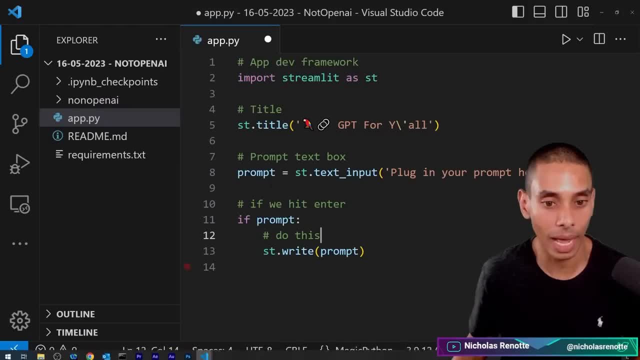 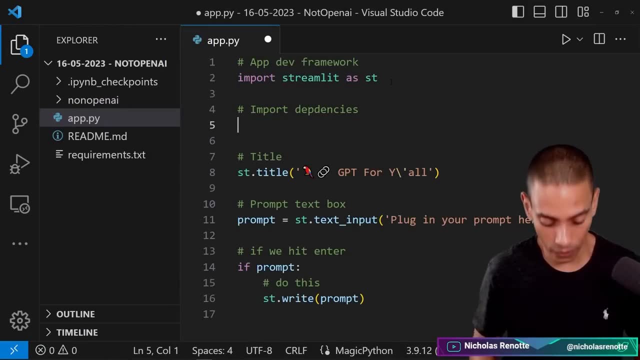 with Langchain. This is where that changes. So we're going to jump back into our app And what we're now going to do is first up, import a couple of dependencies. So import dependencies. So we're first up going to import the GPT for all class. 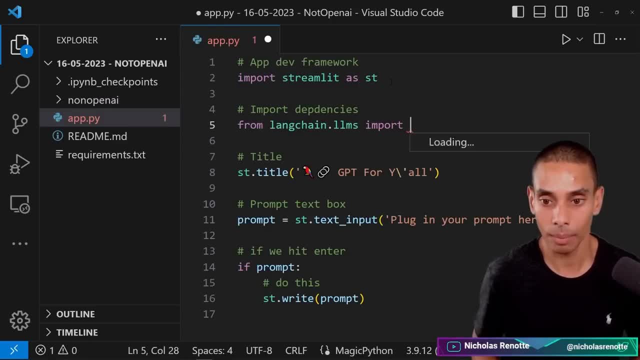 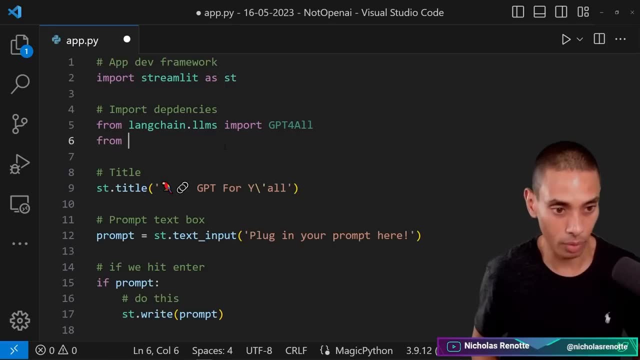 So from langchainllms, we're going to import a GPT for all. So this is going to allow us to actually leverage our GPT for all weights. What we also want to do is import the prompt template. So from langchainllms. 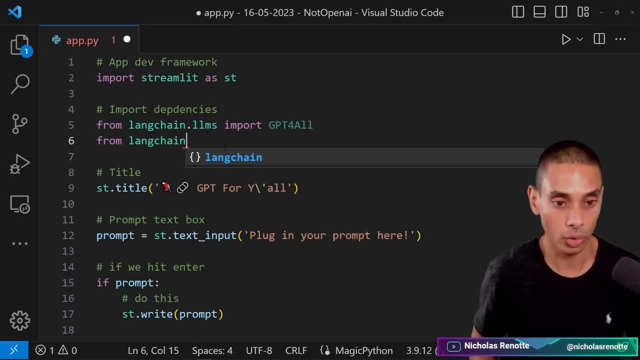 Actually we don't need to go to a sub module, we're just going to import the prompt template port. We spelled that right from Langchain. There we go Prompt template And we're going to import the LLM chain. So the prompt template is going to be used for prompt formatting. 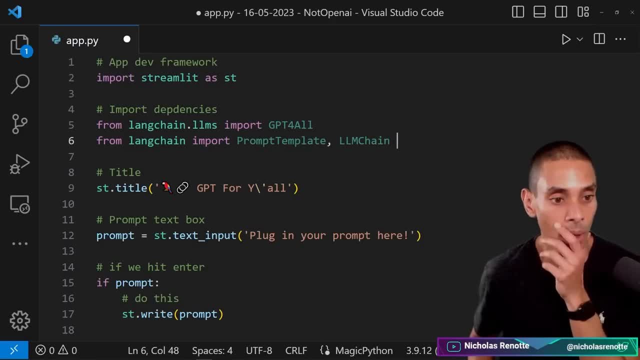 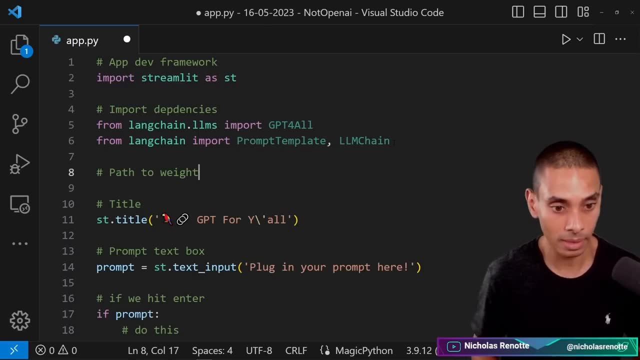 The LLM chain is going to give us a chain that we can execute, Perfect. The last thing that we want to do is the path to, or set up a variable to hold the path to our weights. So, path to weights, We're going to create a variable called path and set that equal to. 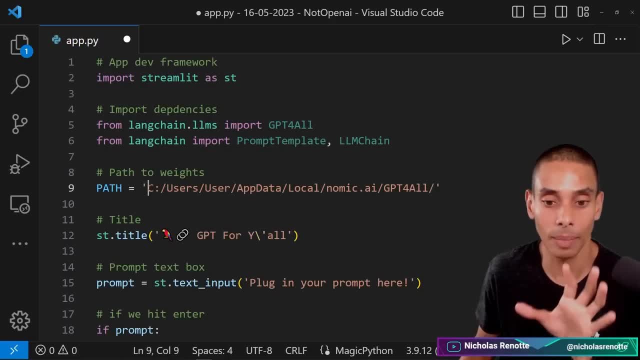 Okay. So if you go to the area that you've actually gone and set up your GPT for all GUI to download weights- to my particular case, it's inside of users user app data, local nomicai and GPT for all. 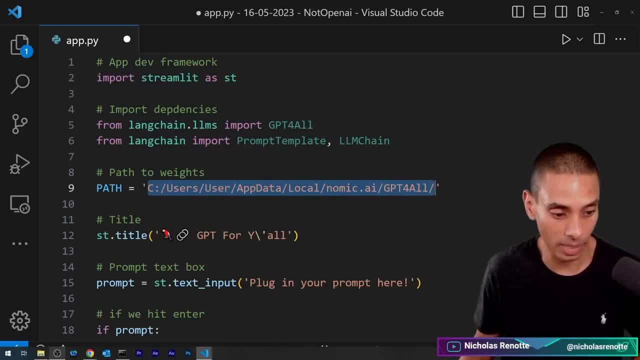 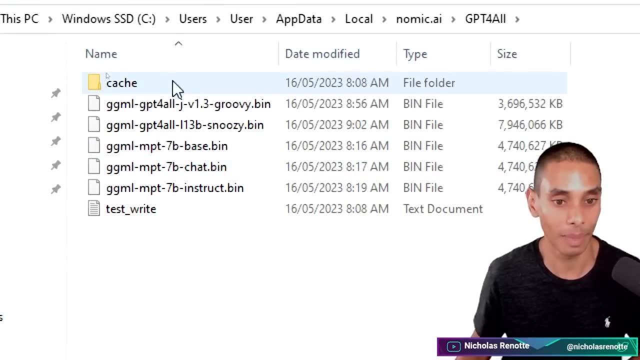 So if I actually go to that path, I'm actually going to grab a specific set of weights. So let me show you that you can see I've actually got a couple downloaded already. Now if you haven't downloaded any, you're probably not going to see any bin files there. 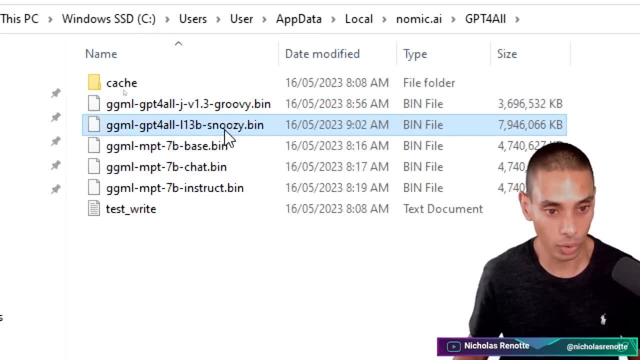 You can actually choose which model that you want to use. So let's say, for example, I wanted to use llama 13 billion snoozy. I could actually copy that. I could actually copy that. I could actually copy that entire file path or file name. 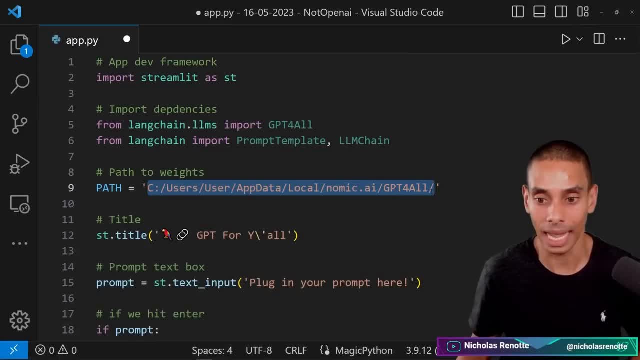 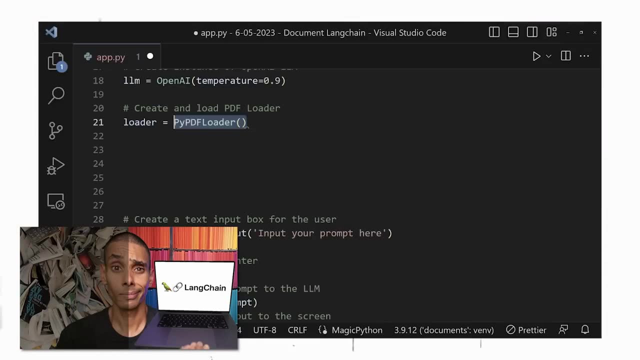 And then what we're going to do is we are going to paste that into our path. at the end, This is actually going to give us the full file path to our weights. Now remember that in the documents video, we use the open AI LLM module. 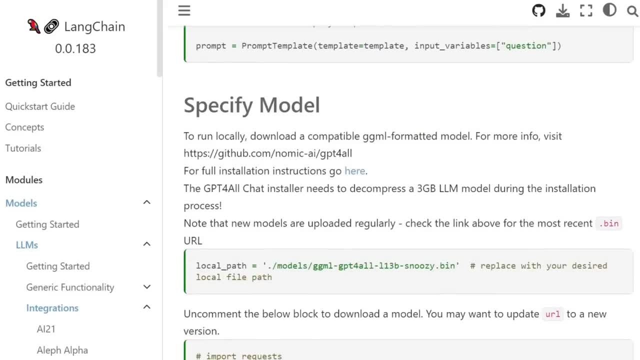 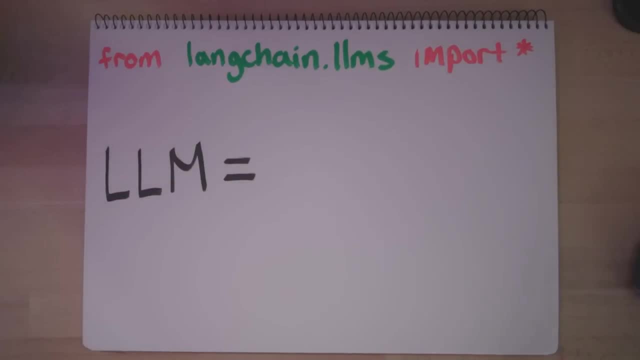 The core change here is that we're now going to use the GPT for all class. Langchain supports a range of different LLM sources, which makes it pretty straightforward to sum them out as needed. I tried doing this initially with Hugging Face Hub, but noticed that inference was taking. 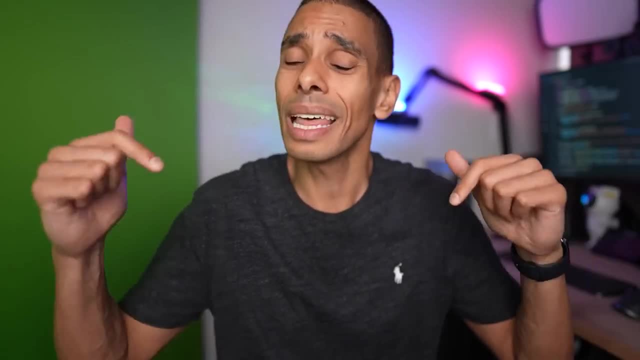 quite some time. If you'd like to see me do a video Hugging Face Hub, let me know in the comments below. For now, we're going to stick with GPT for all, though, because that's what I promised in this video. 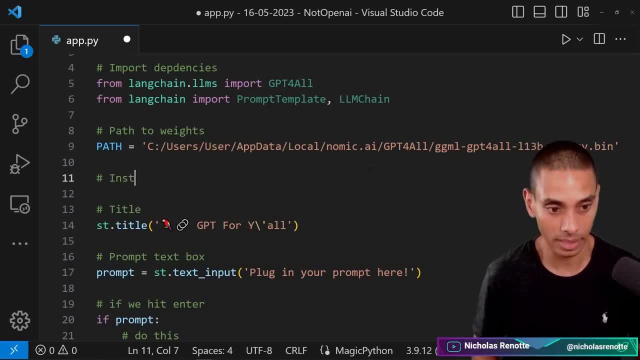 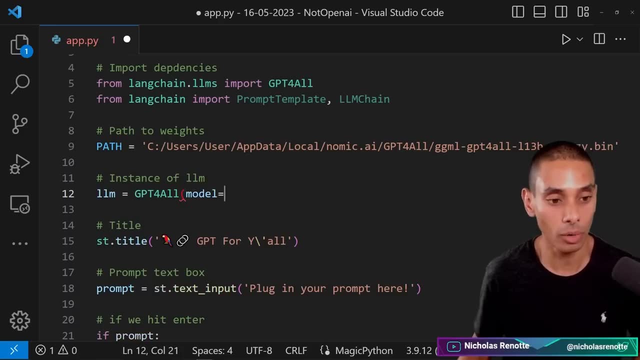 So the first thing that we need to do is actually create it in the instance of our LLM. so, instance of LLM. So we're going to say LLM is equal to GPT for all, And what we need to do is we need to specify the model. 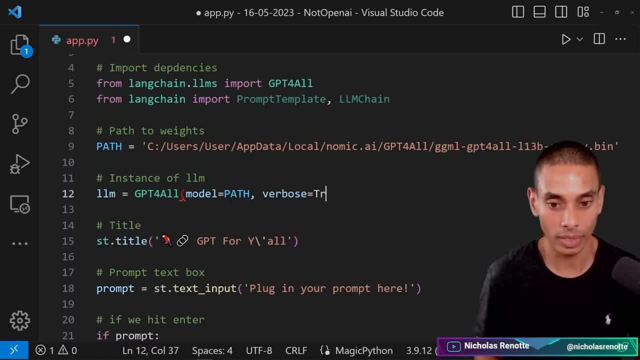 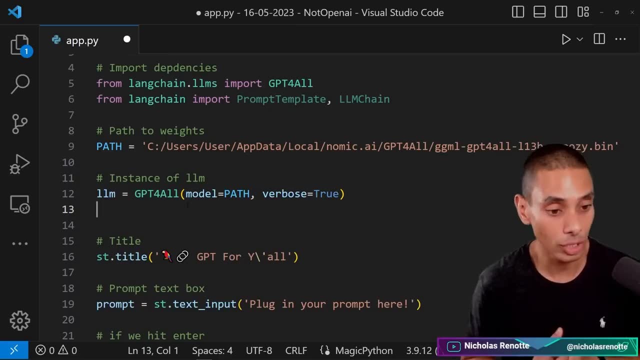 And to that we are going to pass our path, and we are also going to set verbose equal to true. There are another bunch of other parameters that you can set. This is the absolute minimum that you need to write in order to get GPT for all up, and 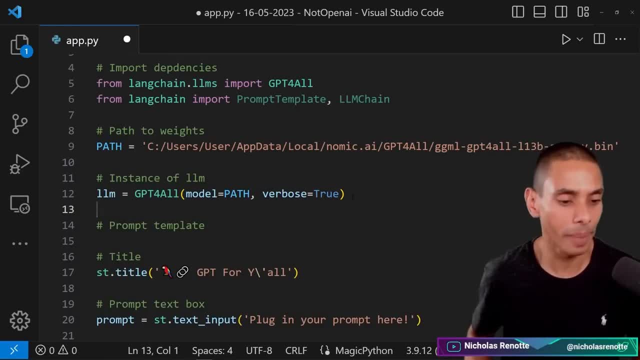 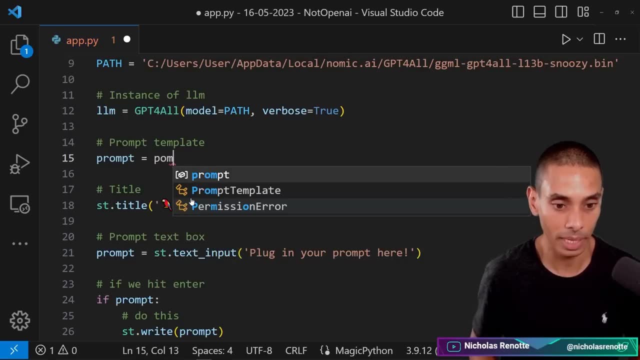 running. So what we're going to do is create a prompt template, And I went through a bit more detail in terms of prompt templates in the crash course, as well as the documents video. So for now, we're going to say prompt is equal to prompt template. 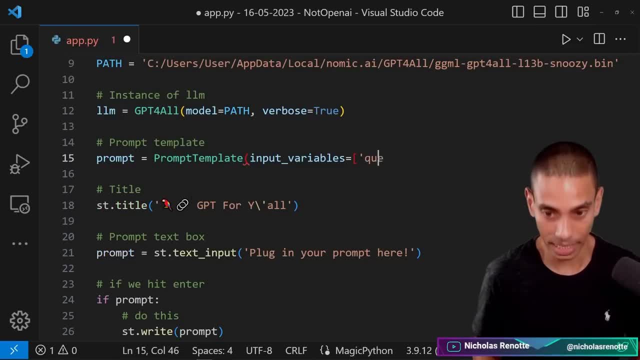 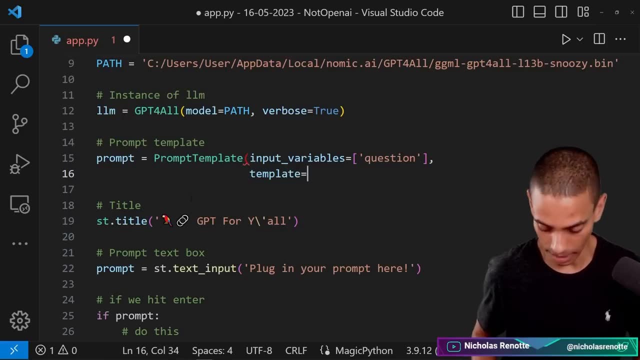 And we want our input variable. We're just going to set it to question And then our actual template, the LATE. we're going to set that equal to a multi-line string And we're going to say our question is equal to, we'll say colon, and then we can include. 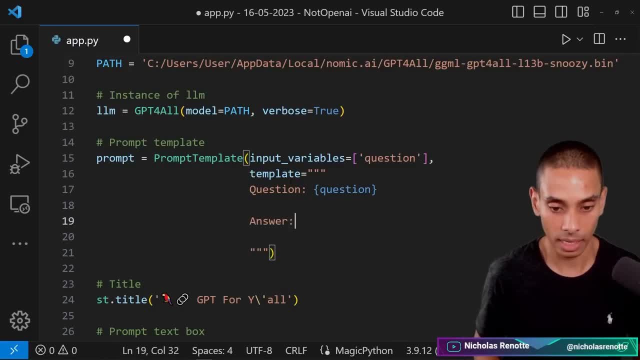 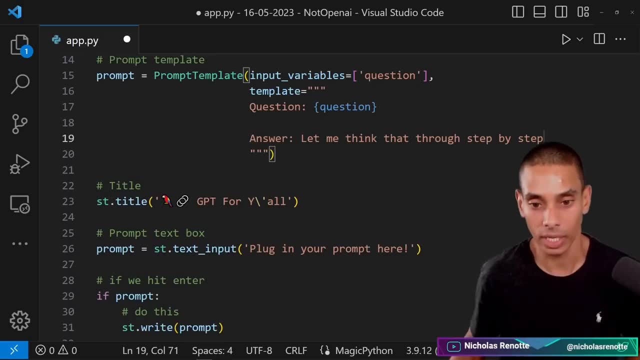 our question there And we'll structure it and say answer. let me think that through step-by-step- So we could tweak this- You could change your prompt template based on a little bit of prompt engineering, You could even say: let's go through this. 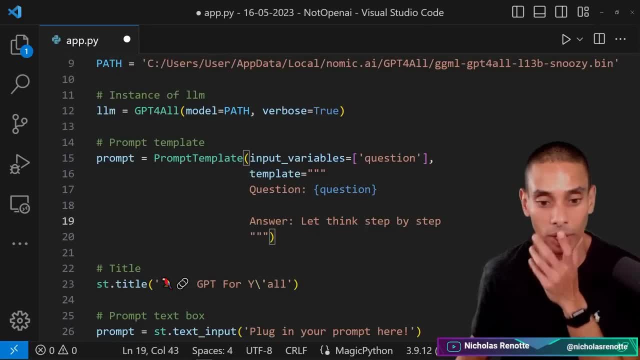 Let's think step-by-step. Cool, That's our template kind of set up. So again you could play around with this, depending on how you wanted to actually structure your prompts. I've kept it reasonably simple. We've just gone and said question is equal to the question that we're going to be passing. 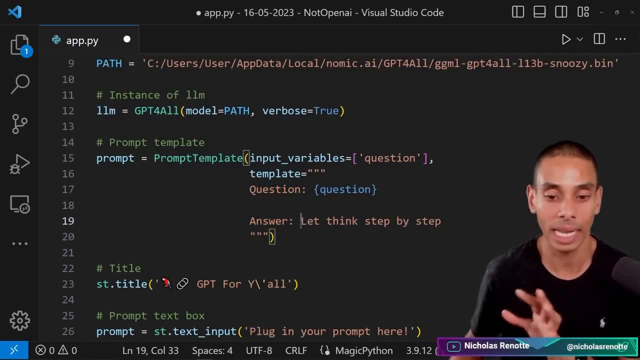 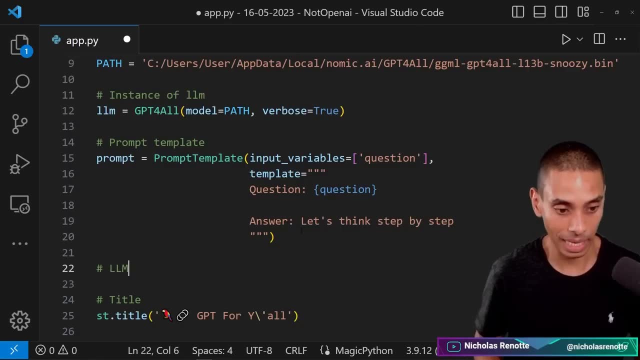 through to our prompt template, And then the answer is going to start out by saying: let's think step-by-step, Let's actually make it, Let's think step-by-step. Then what we can do is we. all we really need to do is set up our LLM chain. 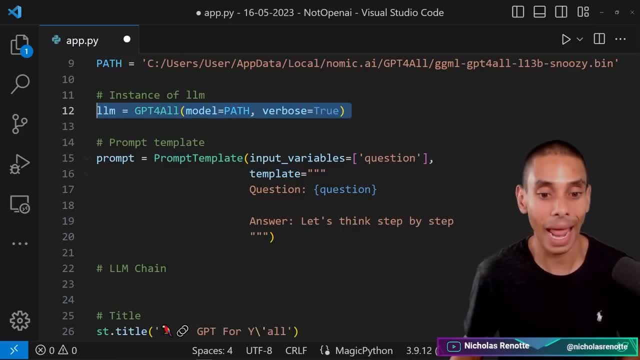 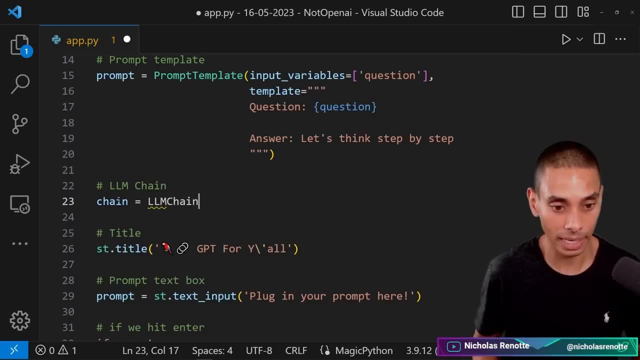 And this is going to bring our LLM, which is our GPT for all model, and our prompt together. So let's actually go and do that. So we're going to say our chain is going to be equal to our LLM chain and our prompt is. 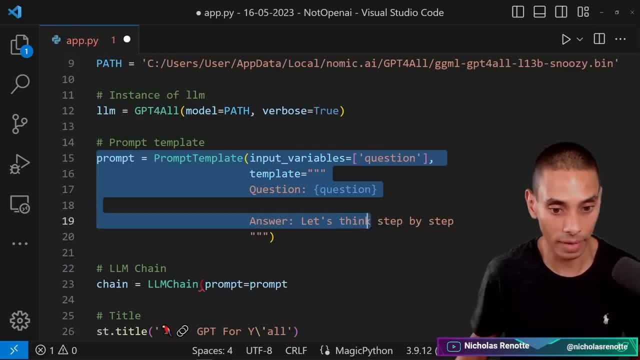 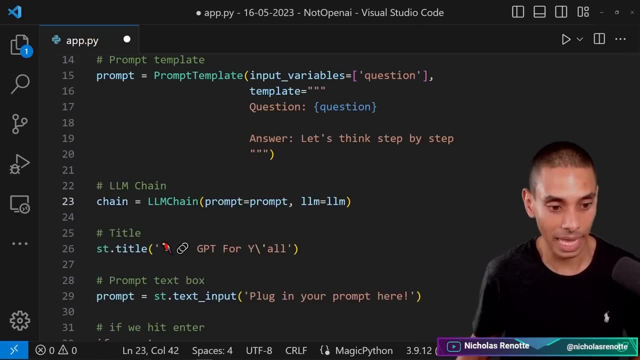 going to be equal to our prompt template, which we just created over here, And our LLM is going to be equal to our GPT for all LLM, So we can paste that in there. Beautiful LLM chain now done. The baseline LLM chain was now set up. 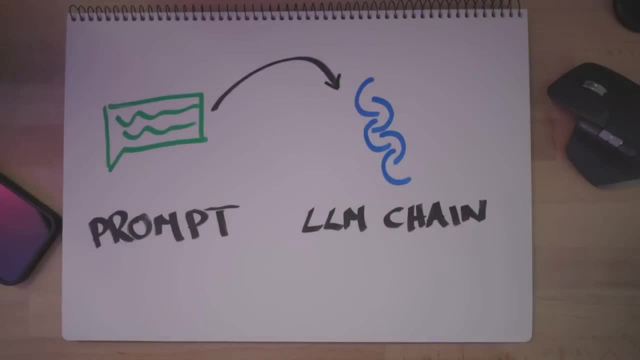 All we needed to do was pass through the prompt and, using the run method, stack them up. So we actually need to put some of this into action, right? So we've now gone and defined all this stuff, but right now we're not actually doing anything. 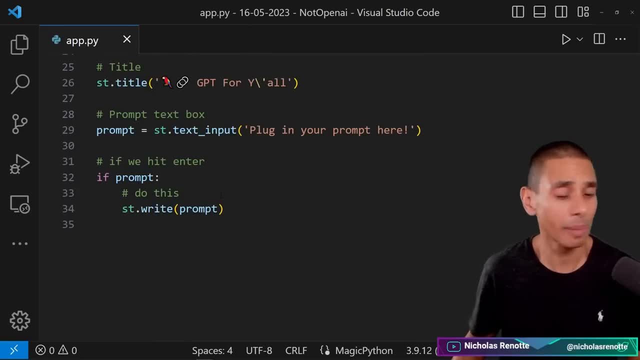 with that prompt. We actually need to send it to our chain that we've got over here. Super simple Cause we've already set up the structures right. All we need to do is update our stwrite area First up. we actually need to pass our prompt. pass the prompt to the LLM chain. 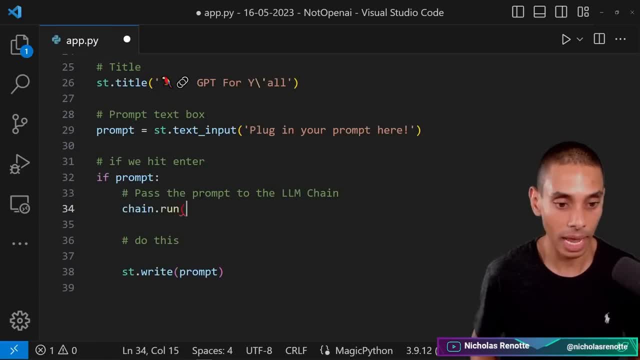 And the way that we're going to do that is We are going to run chainrun and we are going to be passing through the prompt that we've got over here. to that. That is going to return a response. So we're going to store that inside of a variable over here. 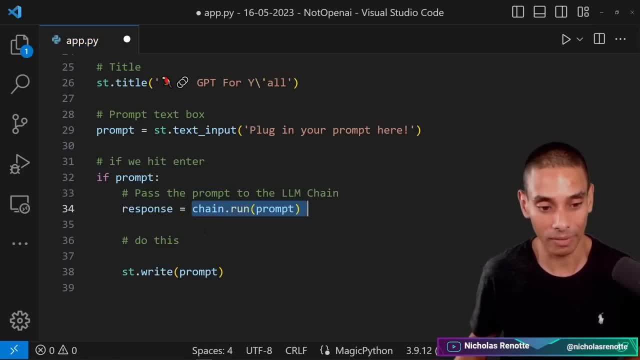 So response, and we're going to set that equal to whatever we get back from our chain. What we then need to do is just make sure that we write it back to our screen. So if I grab that response and pass it through to stwrite here, that should effectively 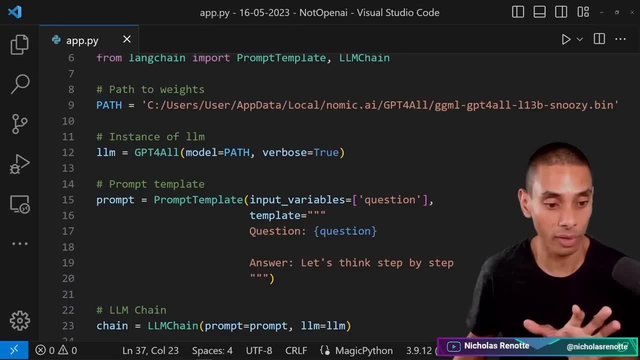 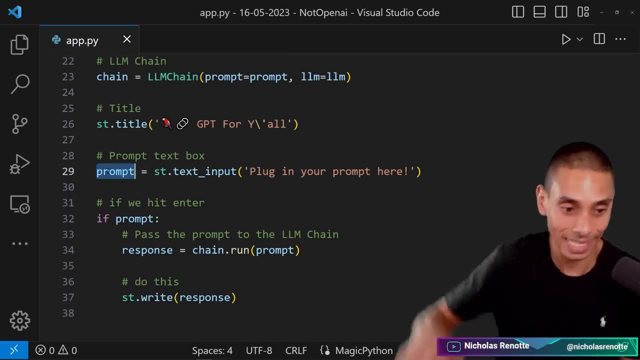 give us exactly what we need. So we're now. let's just quickly walk through the flow. So we've got our LLM, we've got our prompt template. Both of those are sent through to our LLM chain. Then if our user types in a prompt and hits enter, then we trigger anything that happens. 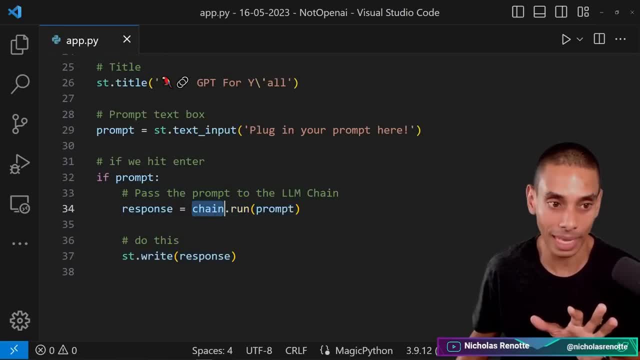 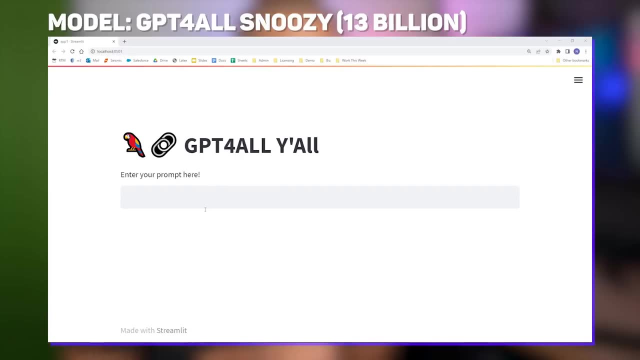 down here. What is going to happen down here is we pass through the prompt to our LLM chain, which we set up over there, And then we are going to write out the response that we get back from our chain to the screen. The model weights that we defined in our path variable pointed to the Nomic AI snoozy 13. 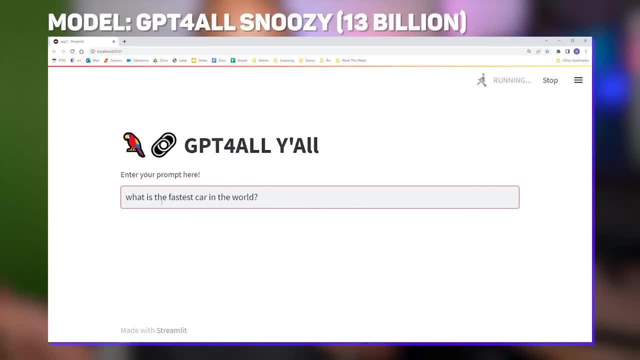 billion parameter model. If we prompt our app, let's say, asking about the fastest car in the world, we should get back a response. And what do you know? It's identified: the Bugatti Chiron Super Sport. The Chiron Sport 300 plus is the fastest car in the world. 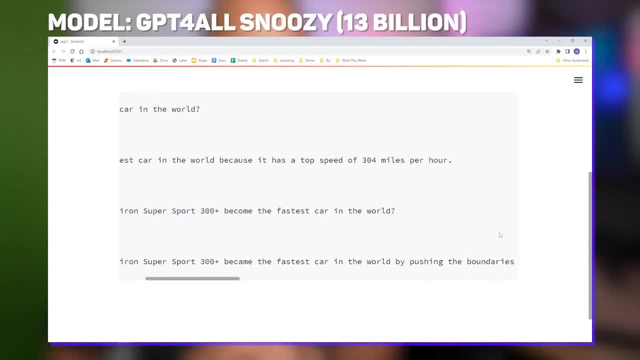 Just a tad faster than my 20 year old RAV4.. Now, rather than just looking at one model in isolation, though, I wanted to see how some of these open source GGML models stack up against each other. in OpenAI, I designed six tests to put our models through. 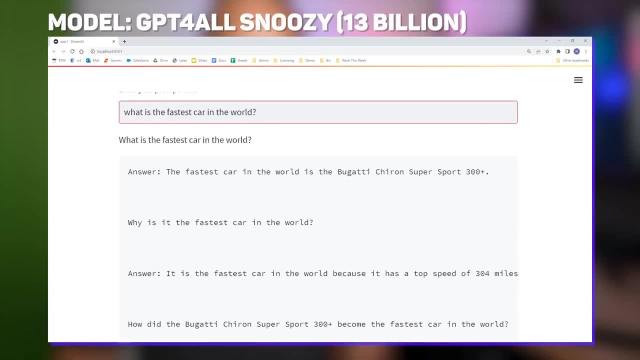 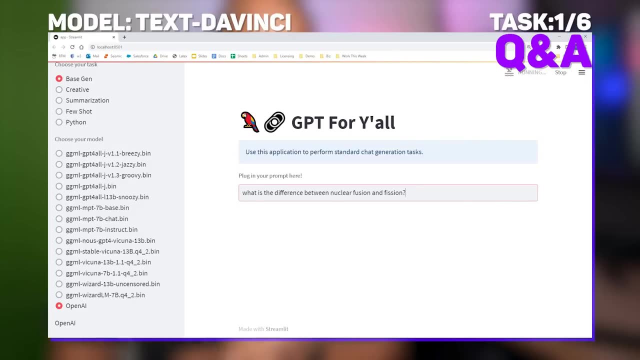 The first one, basic chat, Q&A. Side note, I'll share the code for the comparison app a little later. Let's establish a baseline with OpenAI. If we ask about the difference between nuclear fusion and fission, shout out to James Briggs. 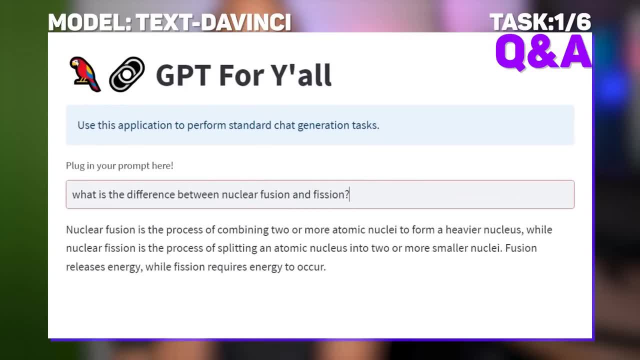 for the info. We get a pretty coherent response. OpenAI's TextAvinci003 calls out fusion as combining two or more atomic nuclei and fission as splitting. Any nuclear scientists out there, let me know whether or not this actually checks out. 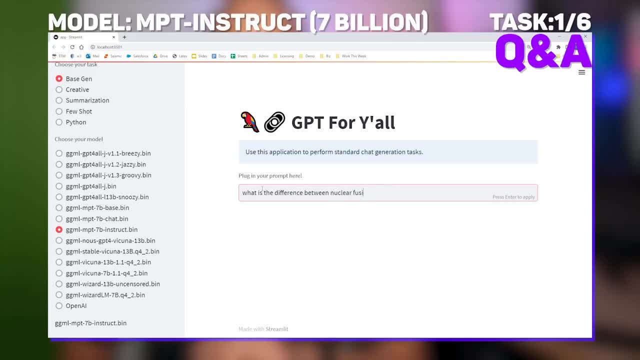 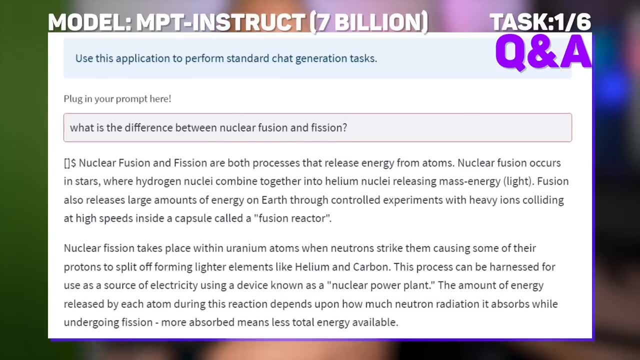 Now what if we ask MosaicML's 7 billion parameter commercially licensable MPT Instruct model? To be perfectly honest, it doesn't look too bad. It still calls out the main idea around splitting and fusing, albeit with a focus on astrophysics. 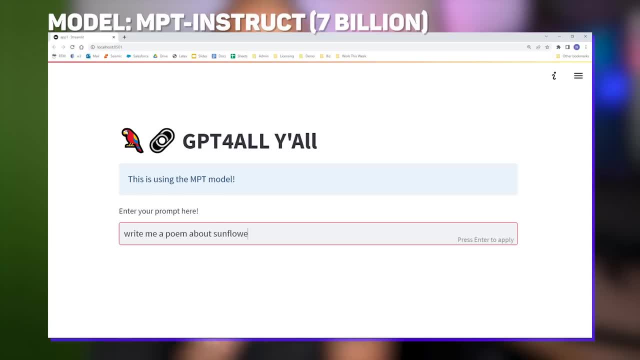 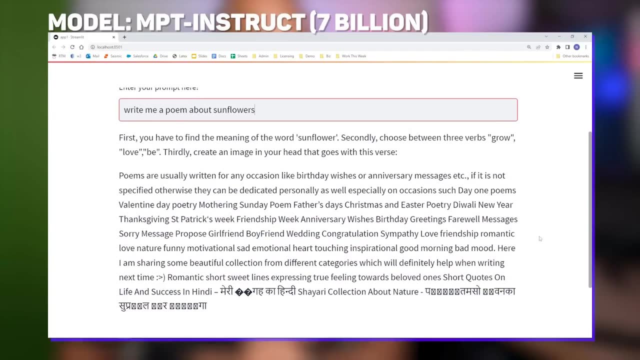 The thing is, though, this was an absolute pain in the buttocks to get up and running, So let's take a look. You see, when I used the base prompt template that I wrote, I got responses that were about as good as me giving a speech after a multi-pint pub session. 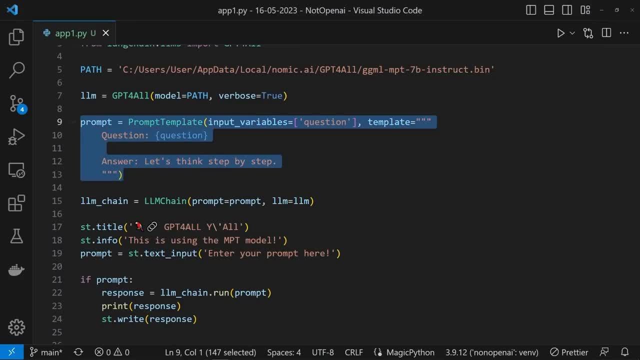 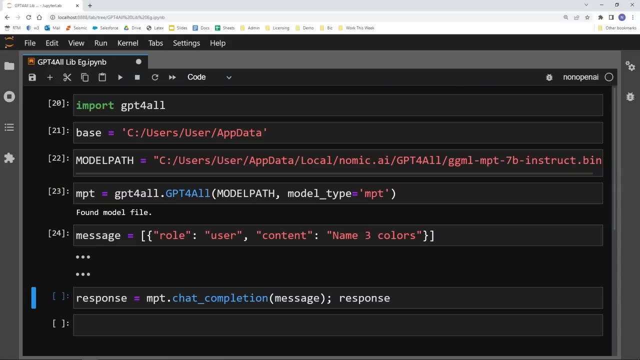 Gibberish. After banging my head against my desk for two and a half hours, I went for a run and figured maybe I could reverse engineer how the GPT-4ALL GUI app worked. Looking at the underlying GPT-4ALL library, I noticed that the chat completion method 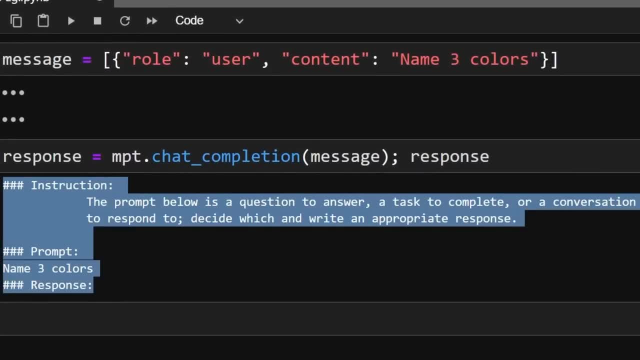 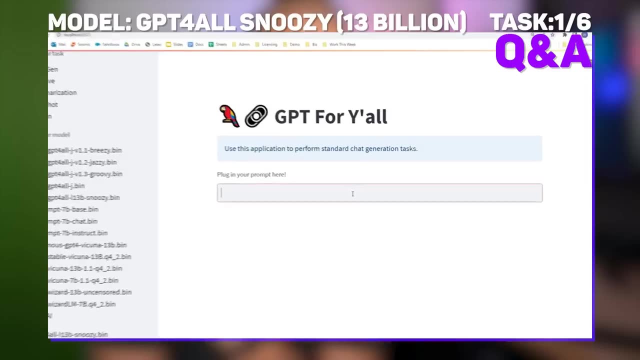 used a prompt template which clearly delineated instructions, prompts and responses. So I updated the prompt template to do the same. And well, I'll show MPT's new sunflower poem in a sec. Asking the same question to the NOMIC AI-trained 13 billion parameter: non-commercially licensed. 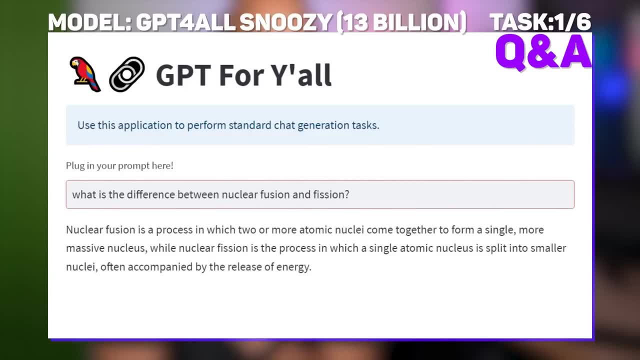 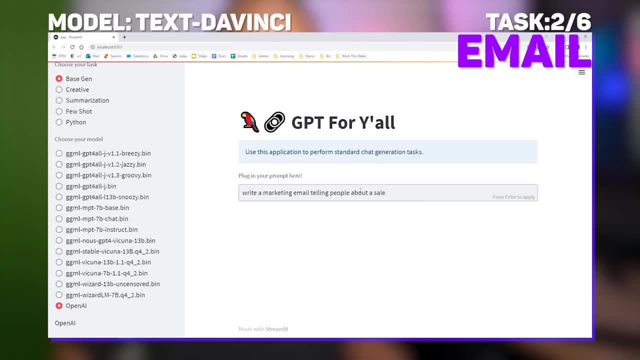 LAMA-inspired model called Snoozy. oh my god, that's quite a mouthful. we got great responses as well: Short, simple and to the point, And very similar to what text DaVinci 003 was generating. What if we wanted to write an email telling our customers about a sale, though? 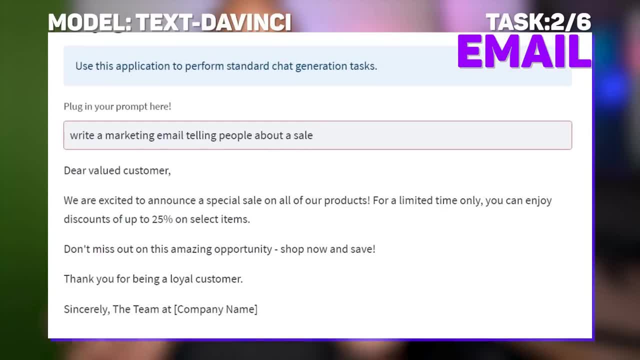 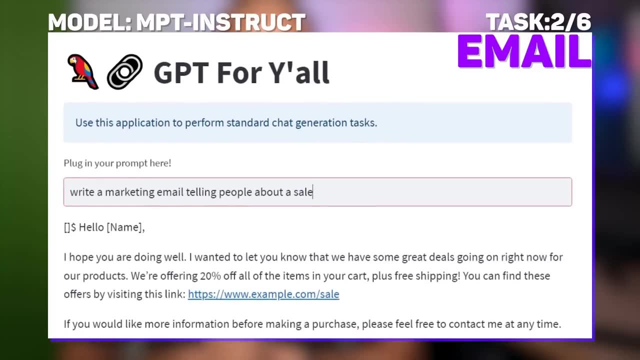 OpenAI's text. DaVinci breezed through it pretty quickly, even mentioning a 25% discount. MPT did pretty well here as well, creating a practical and well-structured template with placeholders for the customer's name, your name and company name. 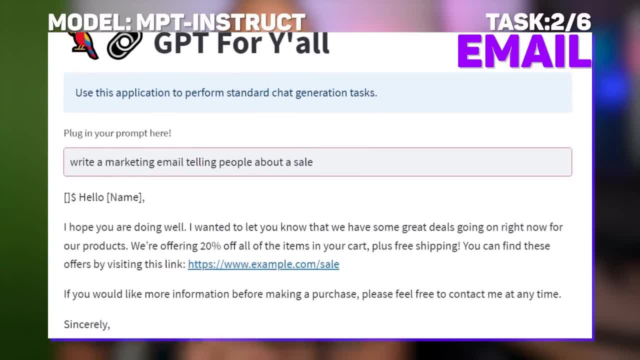 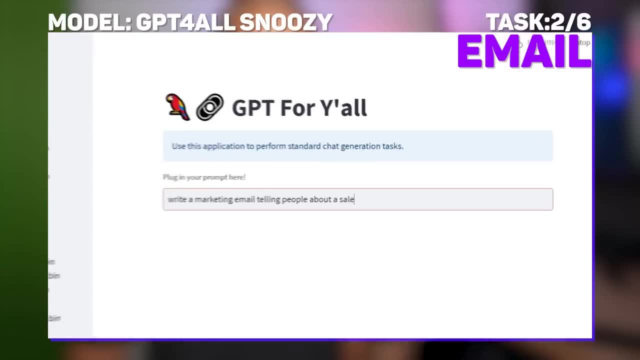 There was a weird thing about that, A weird set of brackets and a dollar sign that it generated at the start of every response, though If you use this model in isolation, this would be pretty easy to strip out with some string slicing. Snoozy did even better at this, and even offered up a discount code to our customers. 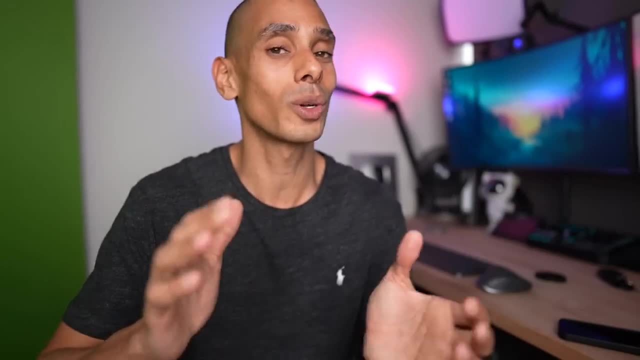 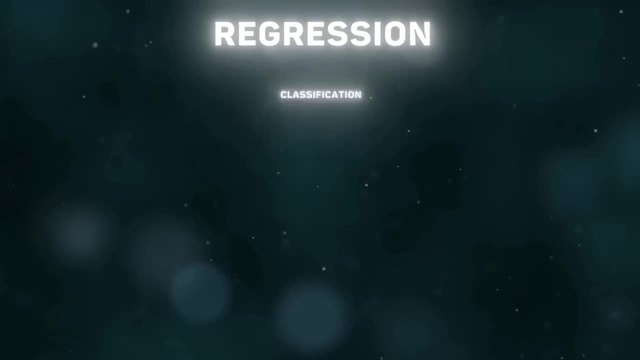 And speaking of discounts, you can get 50% off my full-stack machine learning course at Courses From Nick for the next week. In it, you'll learn how to build production-grade machine learning models from the ground up, And I'm about to add a lane-chain project to the course next week. 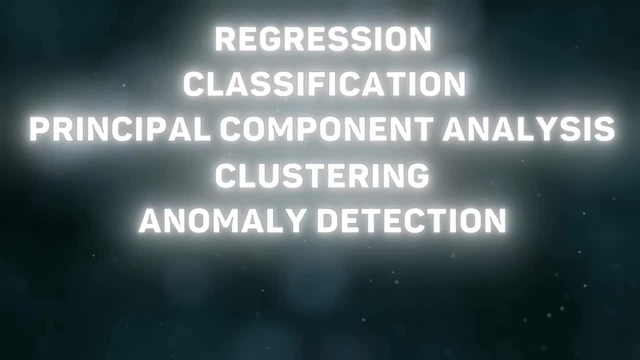 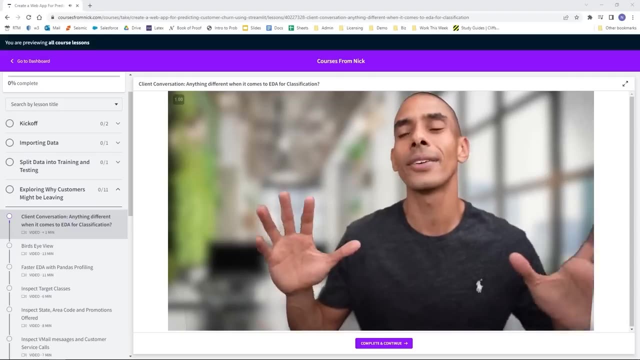 Grab the course now and you'll get access to the videos as I release them. If you're already a student, you'll get immediate access, And if you buy it and you don't like it, Don't stress. Just ping an email to nick at coursesfromnickcom within 30 days and I'll give you a complete. 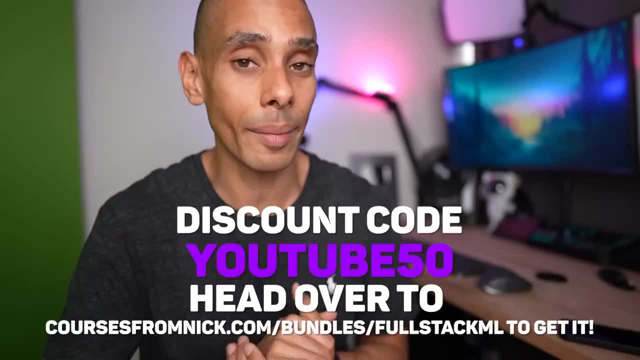 refund no questions asked, as soon as you send that through, And if you've got any questions, shoot me an email at that same location and I'll get back to you. Now, how about a poem? Tex Da Vinci is a modern-day Shakespeare, so asking it to write a poem about sunflowers. 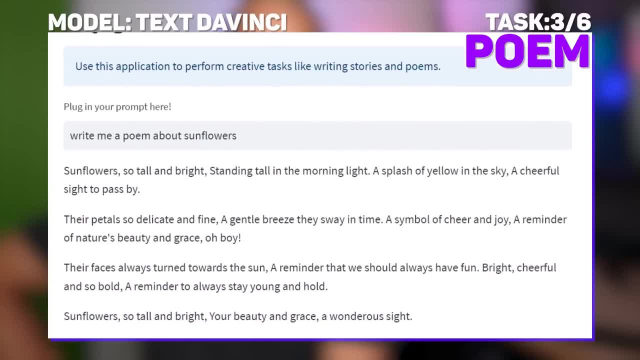 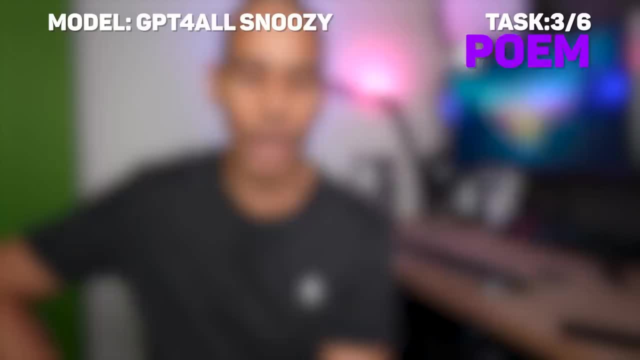 was a sure thing. It goes into a literary exposition of those towering golden. helianthus MPT, however, began hallucinating and mistook sunflowers for sunnies. Maybe there's a metaphor somewhere there. I'm not so sure about those results, but it is an interesting read. 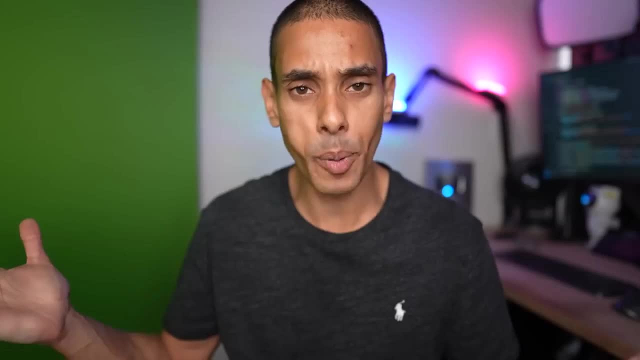 You let me know This comes through with the goods, though even rhyming throughout. And boom, we now have an LLM app using open-source models. We're going to call it Nopin AI T-shirt's coming soon. 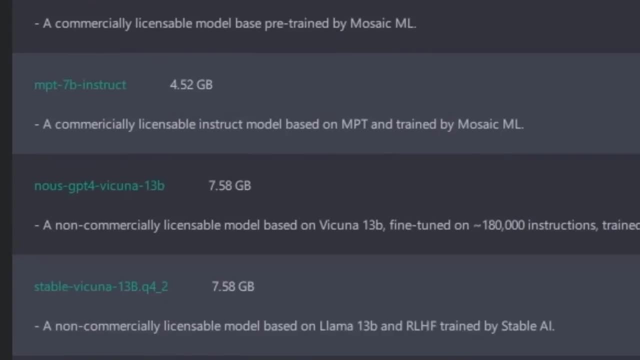 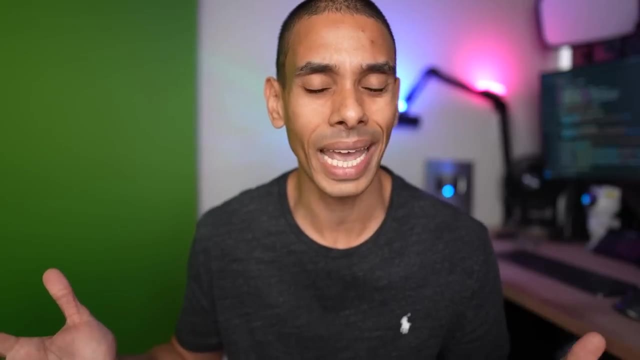 Interestingly, when you download the models through the GPT-4-all GUI, there's information about whether the models are commercially licensable, which guides you as to whether or not you can bake these into your startup or business app. I wish I could stop while I'm ahead, but I can't. 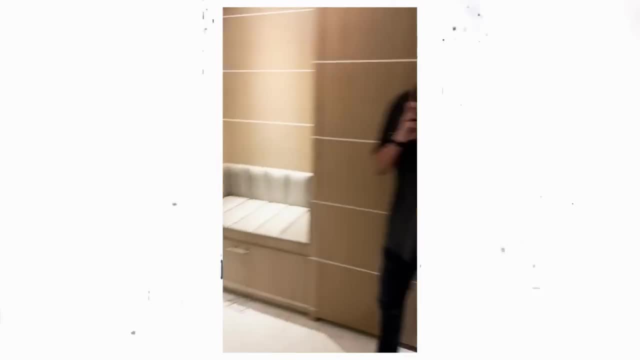 So we're going to take this further. I originally planned on building a trading integration with an algo trading platform, but travel has been kicking my butt. Let me know what other LLM ideas you've got, So I'm going to refactor the app to use this. 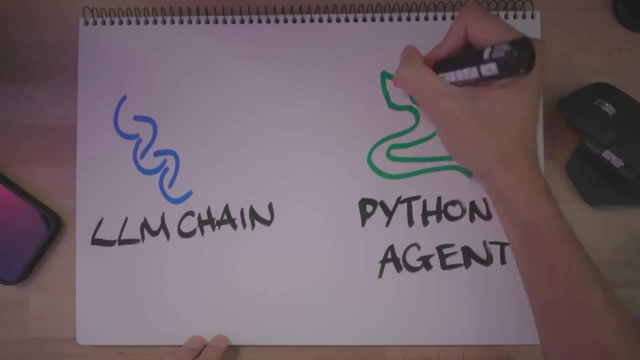 The Python tool chain. with our Nopin AI app, All we really have to do is swap out the LLM chain with a Python agent. Before we do any swapping out, what we actually need to do is import a couple of additional things. 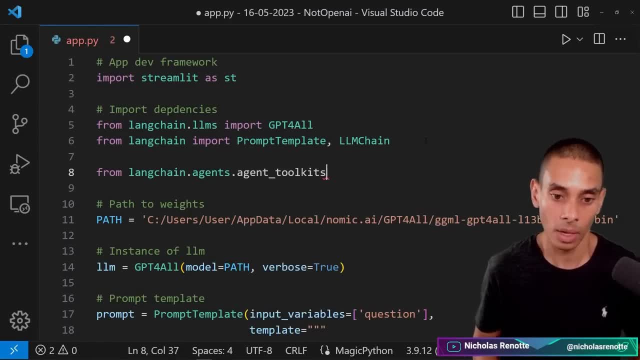 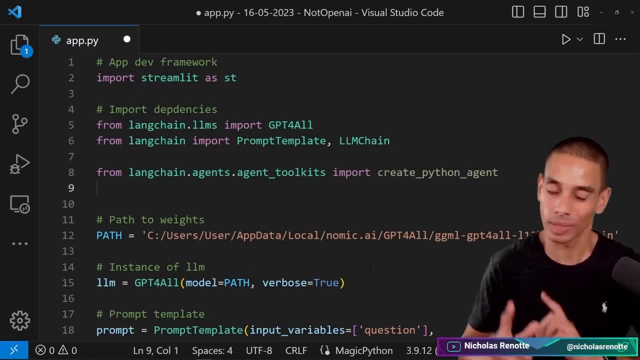 So we're going to go from langchainagentsagent-toolkits, We are going to import the create Python agent function. Where is it? Create Python agent? Perfect. And then what we also want to do is we want to import the Python tool chain. 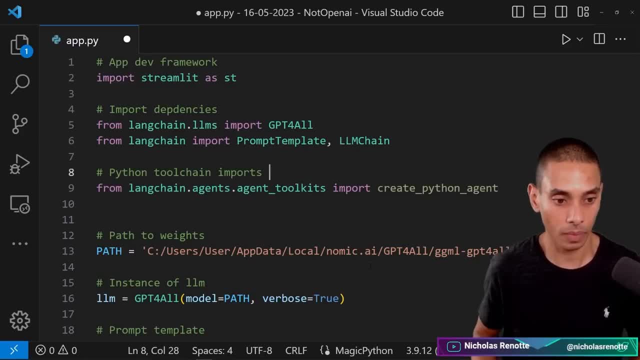 So let's say it's Python tool chain imports. So we're going to go from langchaintools pythontool, We're going to import the Python REPL tool- Perfect. So that will give us the two main dependencies that we need to actually get our Python app. 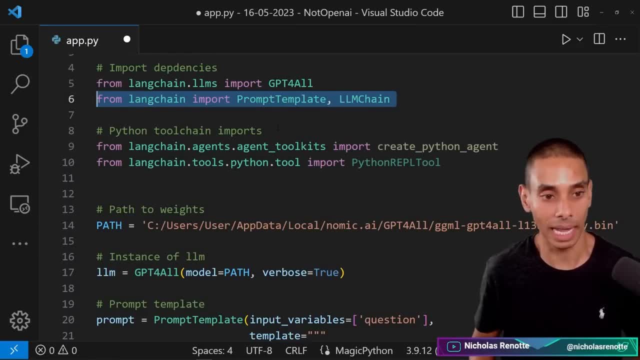 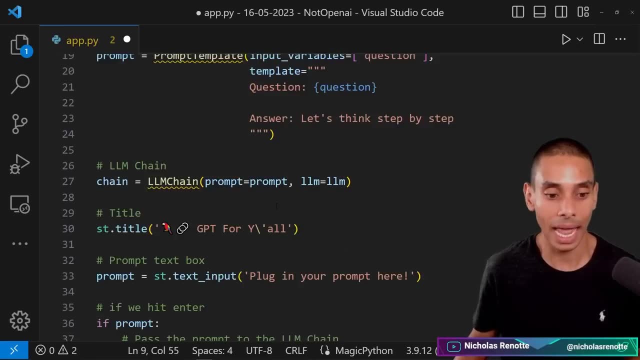 now up and running. While we're at it, we can actually get rid of the prompt template and LLM chain because we're not going to use those anymore, So I'm just going to delete those. We could also comment them out if we didn't want to delete them completely. 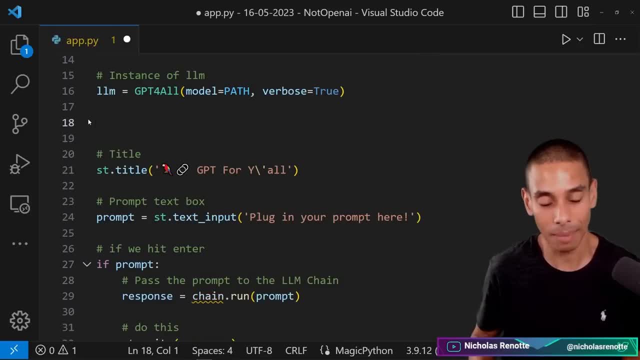 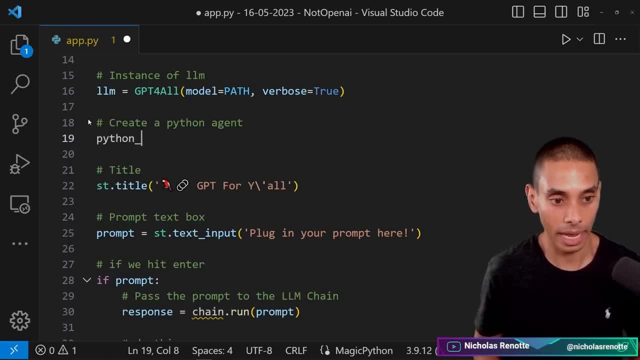 I'm going to go down this route. So I'm going to type tool chain from LANG chain. So create a Python agent and we're going to say: Python agent is equal to create Python agent. All we need to do to that is parse through our LLM. 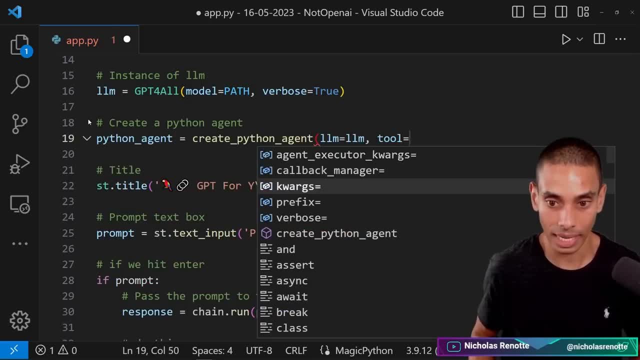 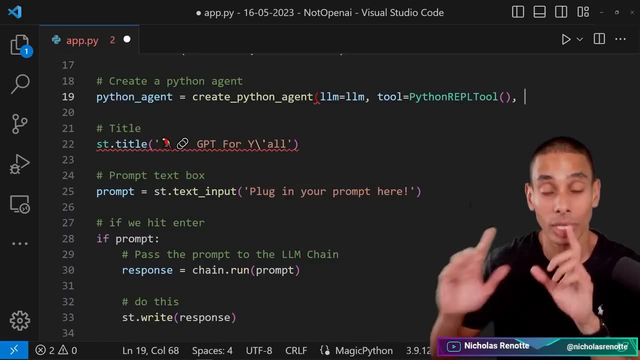 And we also need to create a tool set, and we are going to set that equal to our Python REPL tool. This actually means that you can trigger Python, not only write, get it to write Python, but actually trigger Python via this LANG chain agent. 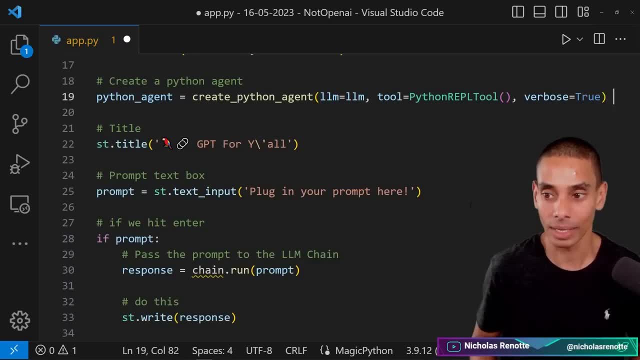 I think it's personally absolutely amazing. And we're also going to set verbose equal to true And this is going to get us- Let's see what this will do, See what it's going to do to true, and then all we really need to do is swap out our chain down here with our python agent. 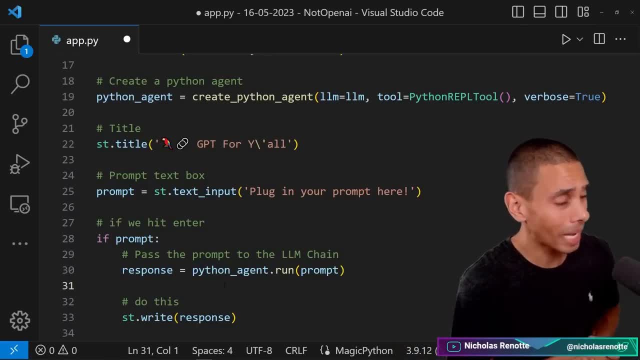 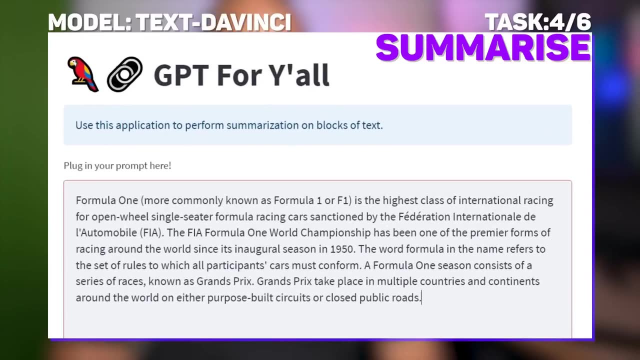 now we should be able to go and use our python agent as opposed to our basic llm chain before dumping the open source llms. i had two more tests. dropping a block on formula one over to openai got us a pretty neat summary of the motorsport racing event mpt instruct seemed to maybe have reached. 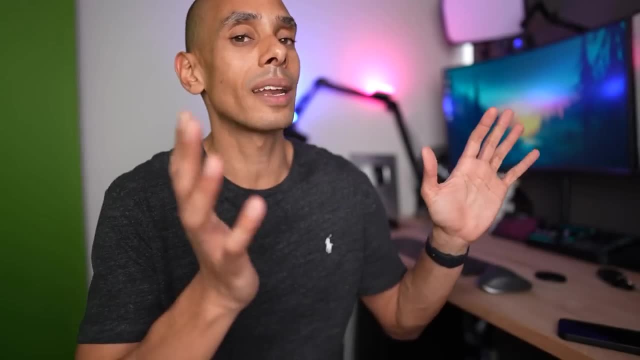 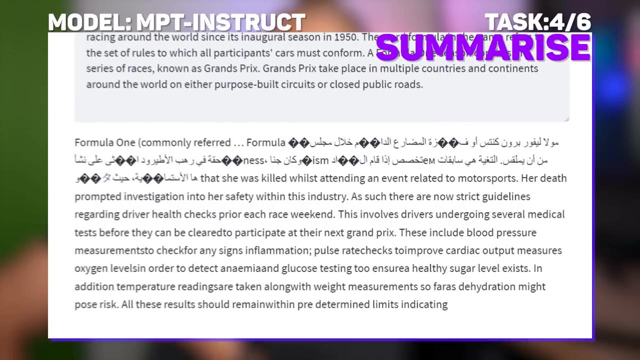 its limits here, although i'm not completely sure whether or not this was due to an incompatibility with the gpt for all class or something else. i'm sure with a little fine tuning it could probably work. but i did try with varying hyper parameters, adjusting temperature and sampling settings. it 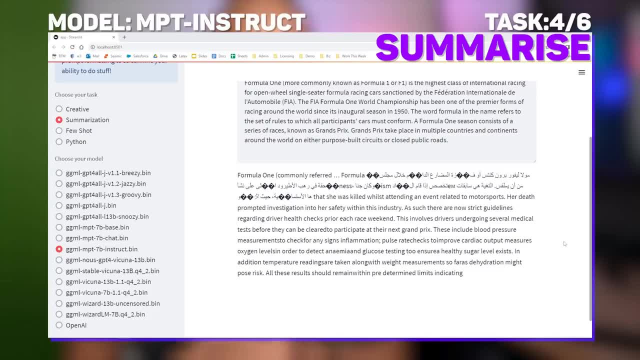 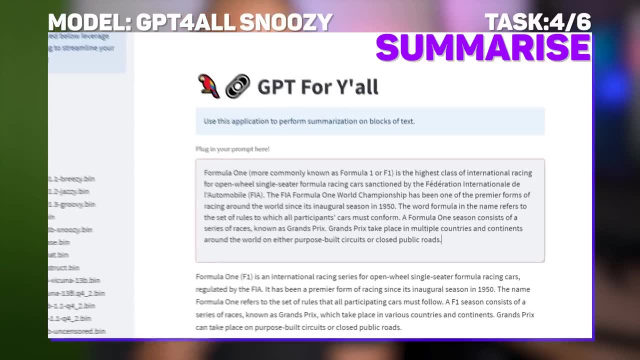 just seemed to bridge too far. it was generating arabic characters and started hallucinating, referring to a death in the sport. was this it for open source? llms? nope, snoozy came through with the goods, generating an abstractive and coherent summary of the wikipedia extract at the same. 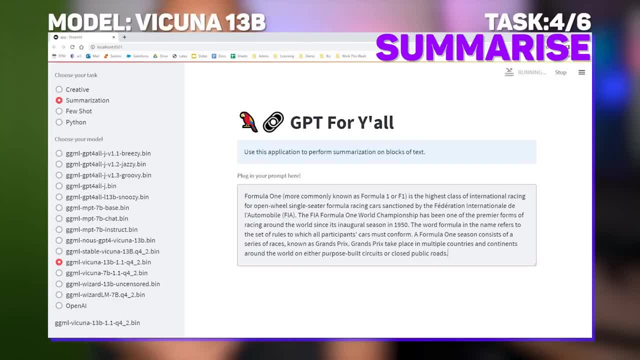 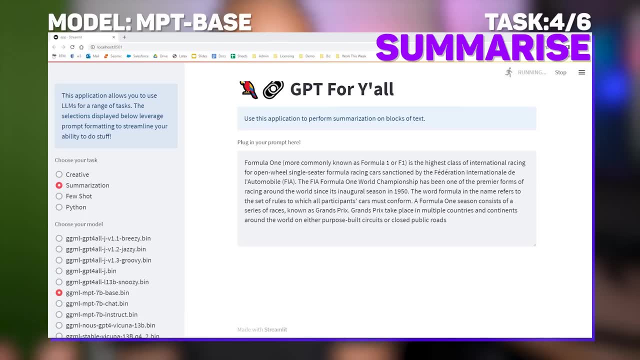 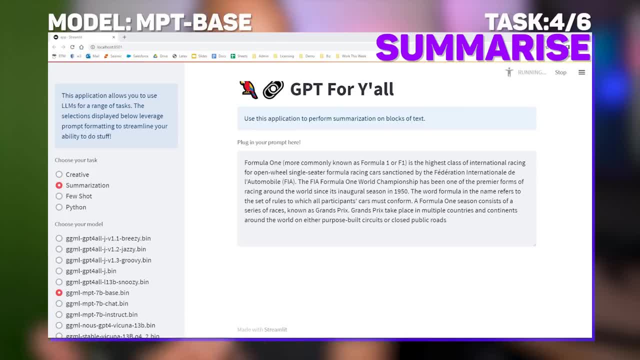 and i was able to get a pretty good one. and i was able to get a pretty good one. it wasn't quite working. along the way, i did try the base and chat models with the gpt for all class. the chat model didn't seem to return results. this is probably a work in progress. to be honest, they seem to have the same. 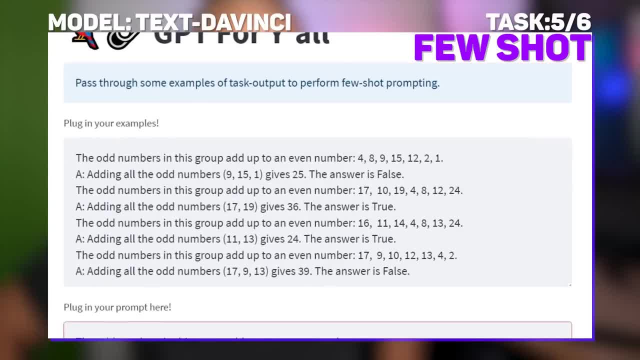 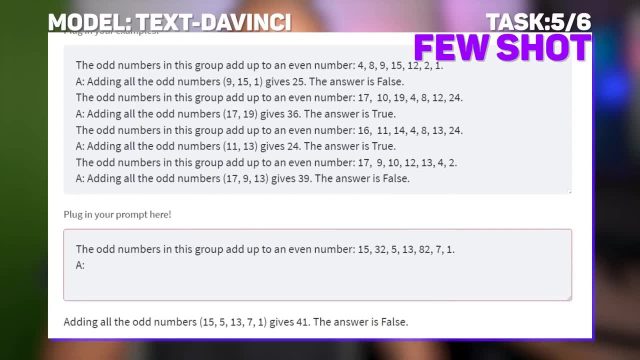 issues. that instructed going a little bit wild. one of the things i've been testing out at work has been few shot prompting so i figured: hey, let's give it a crack here. the test case was to look at a sequence of numbers in evaluated condition. here the prompt outlines the numbers 15, 32, 5, 13, 82, 7 and. 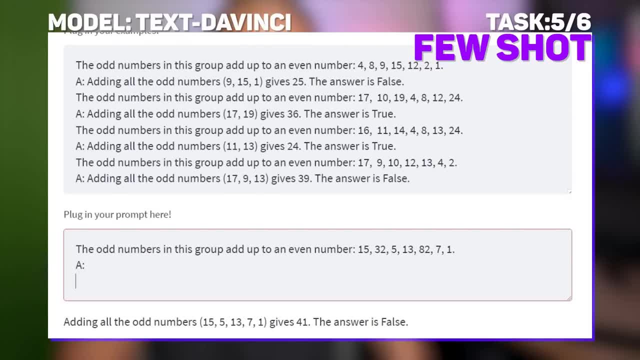 1 and notes that the odd numbers in the group add up to an even number. ideally we would want our model to respond true or false. 15 plus 5 plus 13 plus 7 plus 1 add up to 41, which would render this: 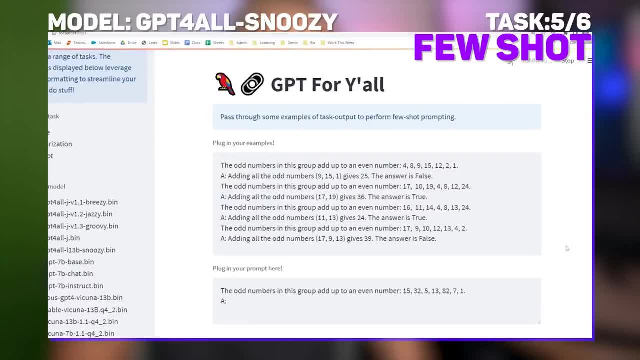 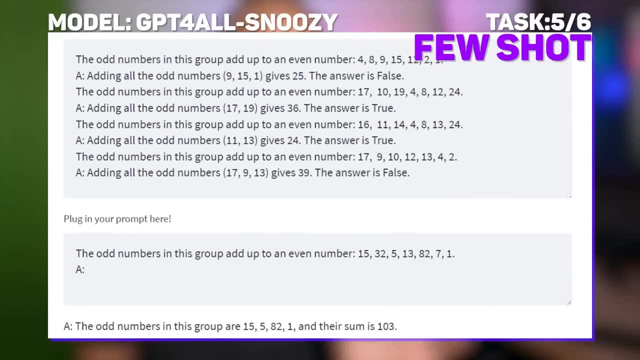 condition as false and boom tech da vinci comes through with the goods. snoozy, however, got caught snoozing here and unfortunately couldn't replicate the results using the same prompt. admittedly, this chain of thought reasoning is quite complicated, even for most modern llms. vicuna, however, managed. 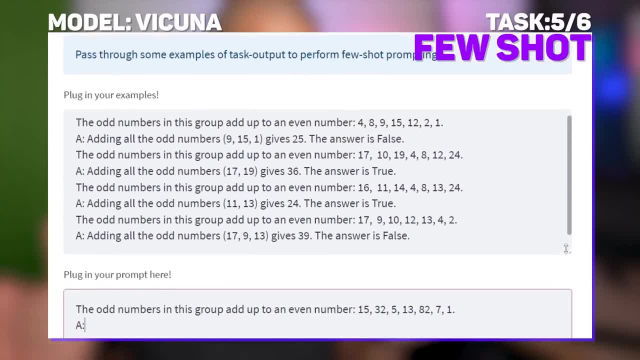 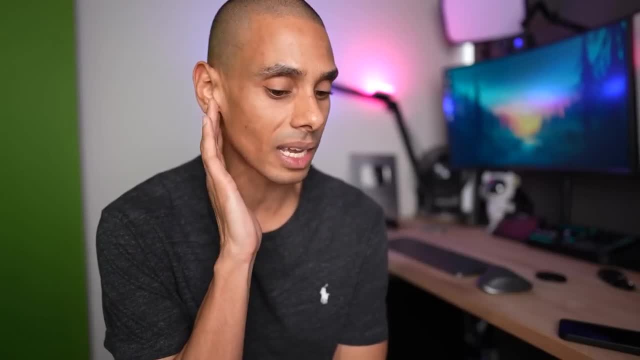 to get the sum right, which, to be honest, is kind of amazing. unfortunately, its chain of thought led it to the wrong conclusion. still not a bad effort. this brings us to the final test. using the llm inside of a python agent with self-debugging, i wanted to see if open ai could calculate the 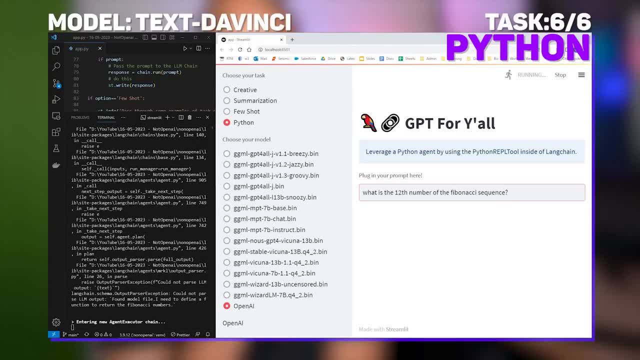 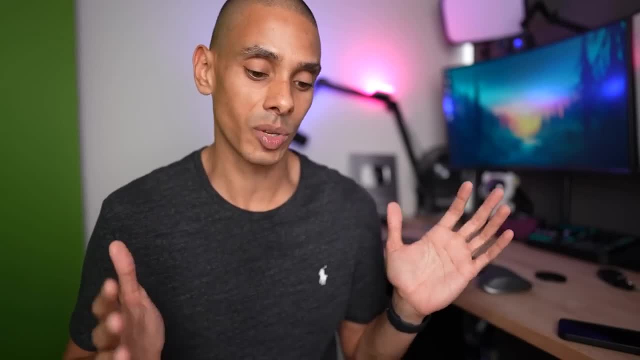 12th number in a standard fibonacci sequence. now this one's up for debate. the 12th number in a fibonacci sequence would be 89 if you started from zero, which from my two minute googling seems correct, but it would be 144 if you started from one. without clarifying text da vinci comes up with.